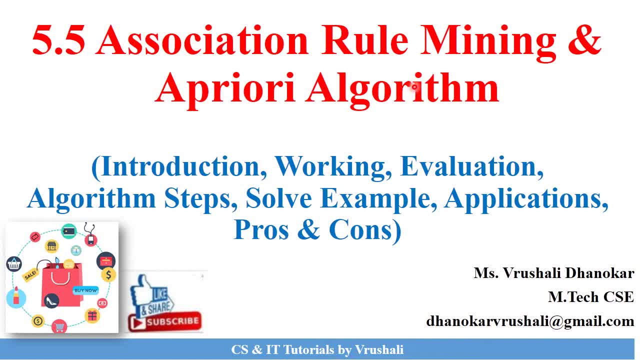 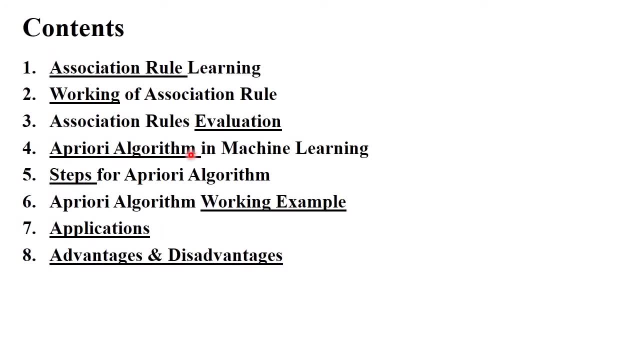 I am going to present the next topic, that is, association rule, mining and a priori algorithm. So let's see, In this session we will discuss about association rule, their working, their evaluation, a priori algorithm, their steps, working, example, applications and advantages. 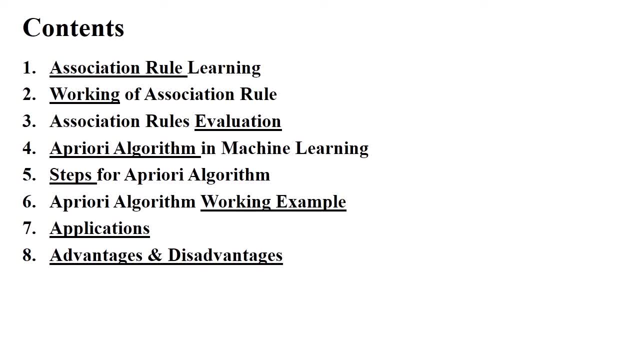 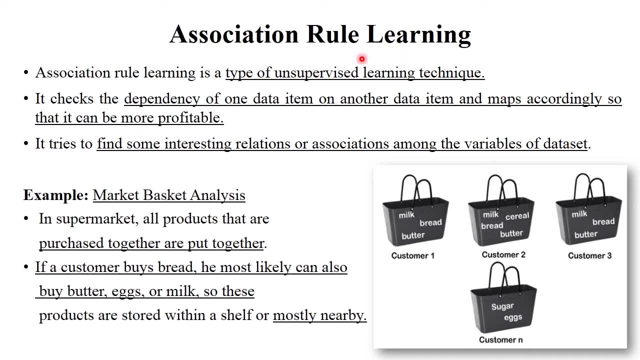 and disadvantages. So let's see one by one. The first point is association rule learning. So basically, this association rule learning is a type of unsupervised learning technique, because it's work on randomization, Random data set. So here let's take one example. The best example of association rule is market. 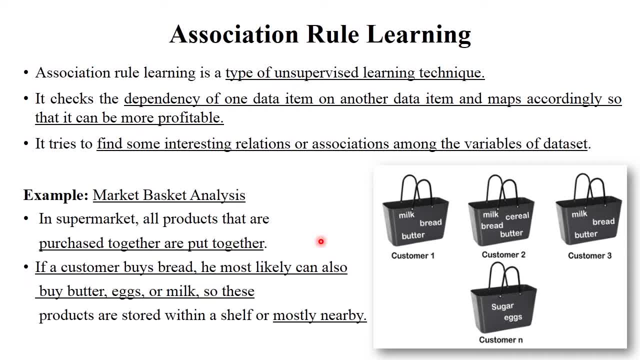 basket analysis, like in any shopping malls or in any mart, where suppose a customer buy a bread, then they also buy a butter, eggs or milk, like this. So this, every things that purchase together are put together right. For example, customer one: they buy milk, bread, butter, Then second: 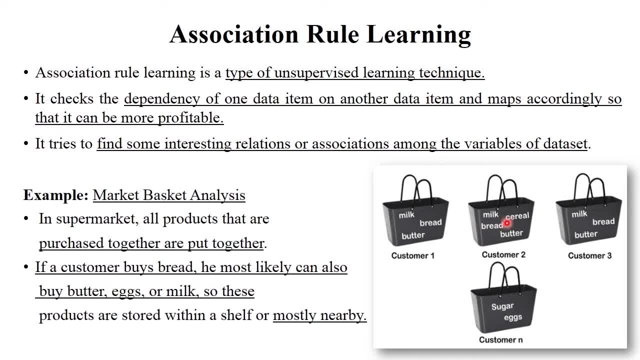 customer. they also buy milk, bread, butter And other related things, Right? So this is called as association rule. Means: suppose person buy a milk, then they also buy a bread, So this concept is called as association concept. So in this association rule it dependency of one data item on another data item. 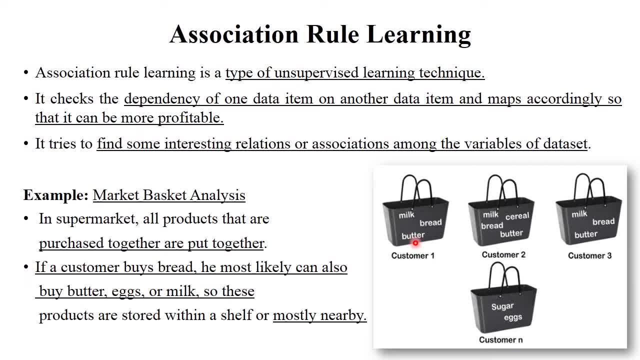 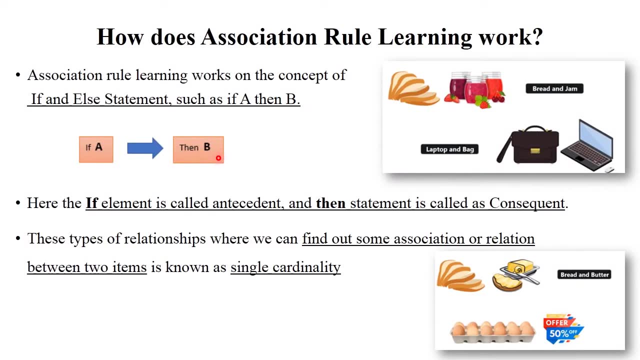 it check that. That's why this all things are put together in any particular supermarket So it find the super interesting relation among the different kind of data set. That's why this association rules are used. next, the next concept is: how does association rule learning work? 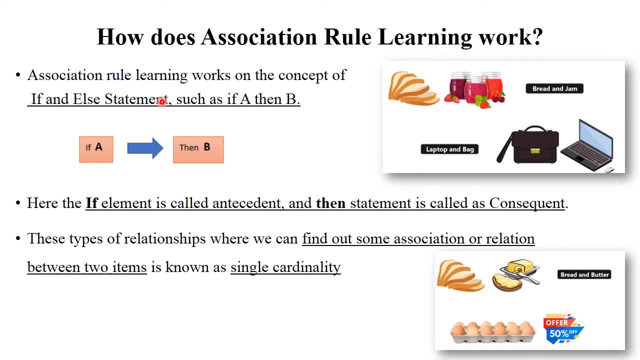 so basically association rule is based on if else statement. for example, if particular person buy a, then they also buy a b. in this way, for example- see here: if a particular person buy a laptop, then they also buy a bag. so this is called as one kind of association rule here, this if element. 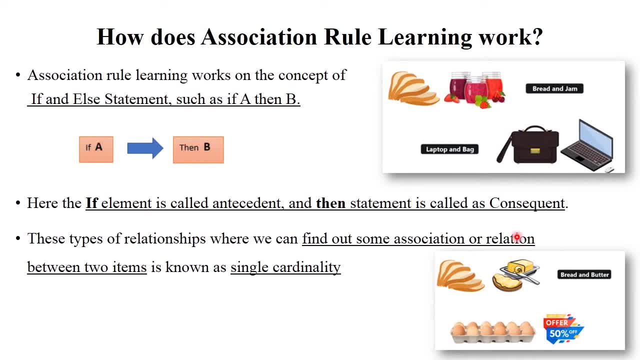 is called as antecedent, and this dan element is called as consequent, and this complete relationship is called as single cardinality, and that's why this kind of rules are used in different supermarkets and these things are more profitable. so another again example is there. if particular customer 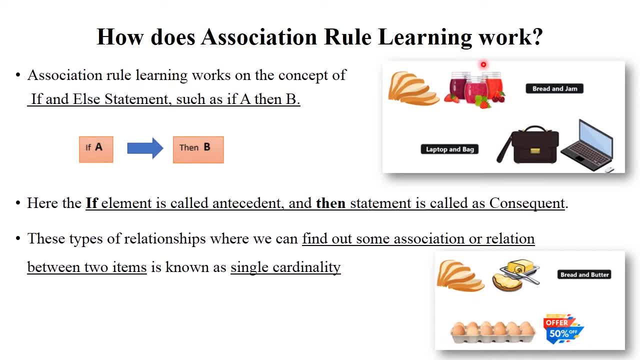 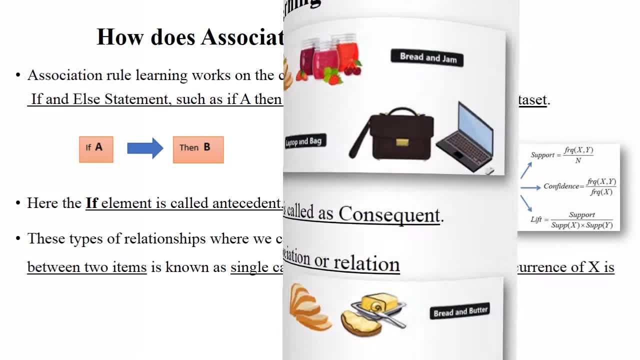 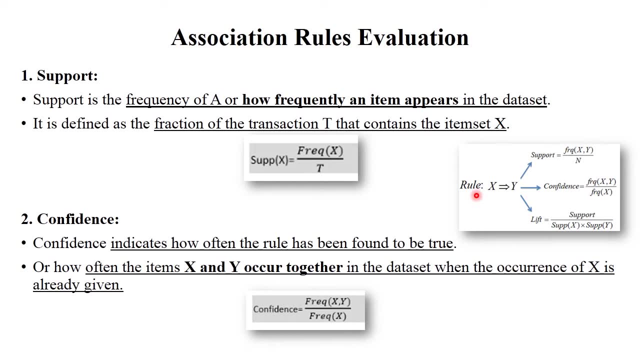 buy bread, then they also buy a jam, right? so these all things are put together and this is called as association rules. next you. so next point is association rules evaluation. so this association rules are calculated by using two concepts: one is support, another one is confidence when we, when we will execute a particular 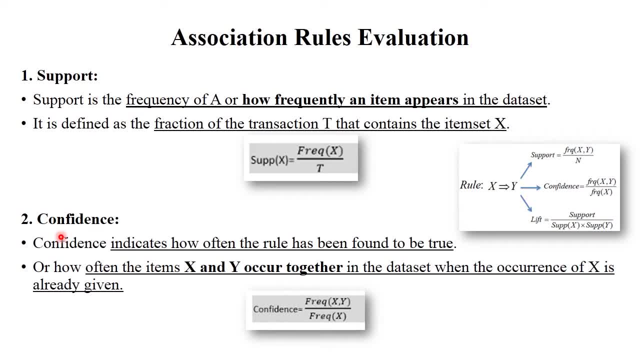 problem statement at that time. in this a priori algorithm, this support and confidence, these two concepts are used for solving the example. the first one is support. what exactly support? support means how frequently an items are appear in data. for example, person a buy milk, then person b. they also buy milk and butter, right? so this two transaction, how many times? 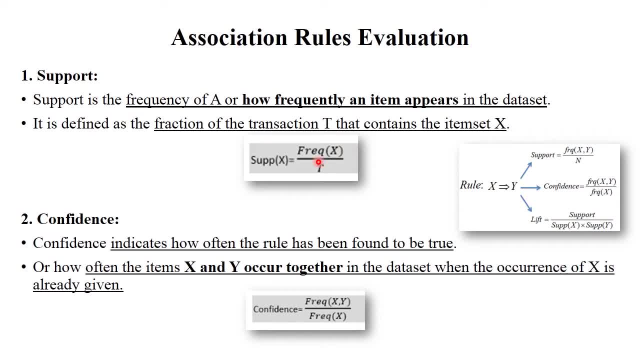 mils are present two times, so this is called as support. means milk: how many times milks are purchased, so this concept is called as support. means the frequency of particular buying item upon transaction, so this is called as support. next one is confidence, so confidence is related to the how many times a particular items are. 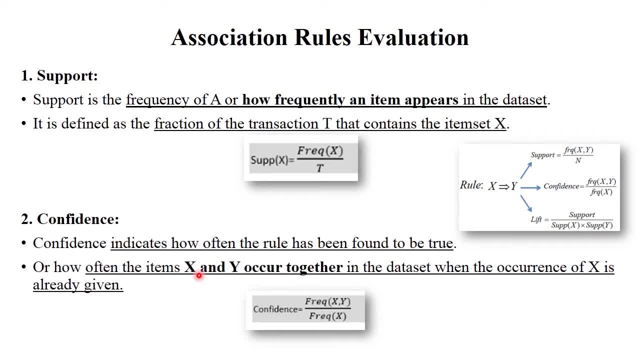 bring together or purchased together, for example, item x and y. so this x and y, this both items are occur together. this is called as confidence Confidence. they check how many times the frequency of that particular purchasing item. So these two terms are used while solving the example support: how many times a particular 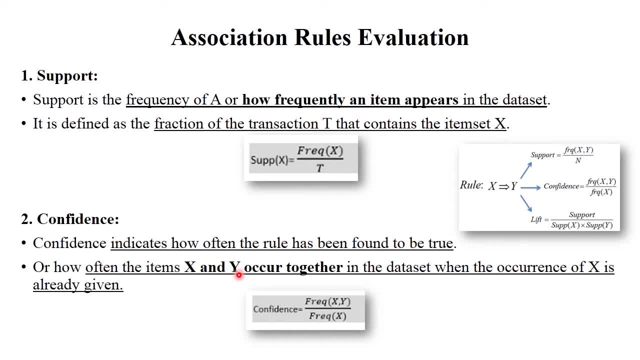 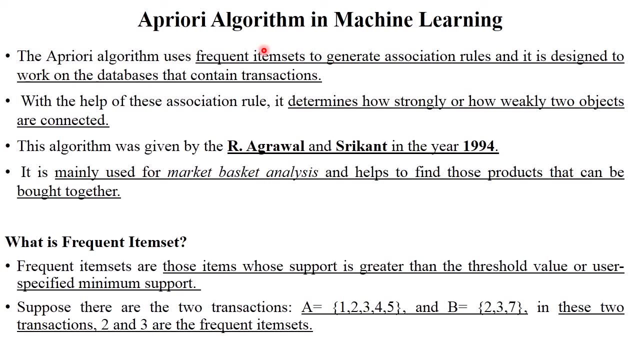 items are purchased- single item and confidence: how many times two items are purchased together. So this is called as confidence. So we will use this formula for solving the example. The next point is a priori algorithm. in machine learning, So a priori algorithm generally used to calculate the association rules by using support and. 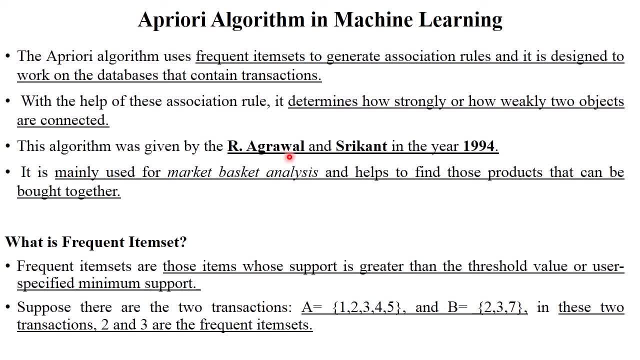 confidence. So this algorithm was developed by R Agarwal and Srikant in the year of 1994.. So basically a priori algorithm is used to calculate the frequent item sets in this market basket analysis. So what exactly frequent item set see here in this term? suppose there are two transaction. 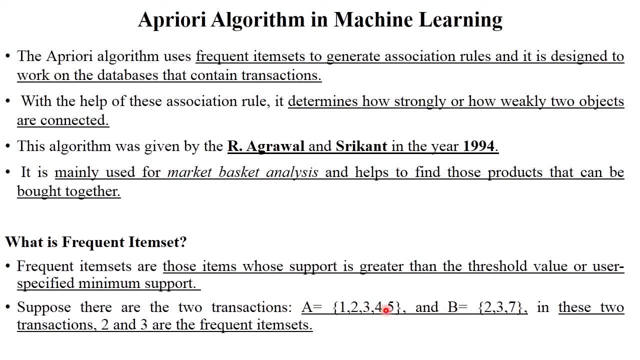 person A purchase one, two, three, four, five items and person B purchase one, two, three, six items and person B purchase one, two, three, five items, right? so this? both person purchased common item, that is, 2 and 3, right? So this is called as frequent item sets. 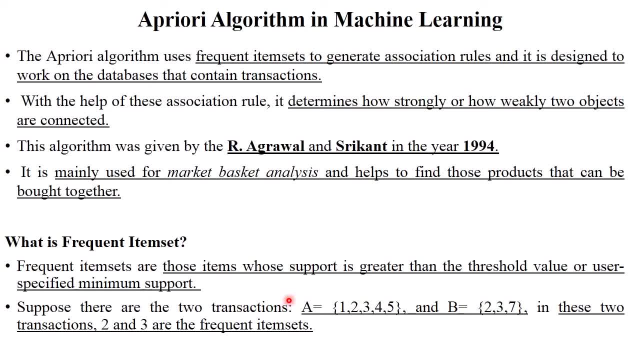 So the items which purchase commonly by using different transactions or different persons, So this is called as frequent item sets. so this a priori algorithm. a priori algorithm generates or determine how strongly and how weakly two objects are connected. For example, majority of that persons are more. this is called as strongly, strongly connection between these two. 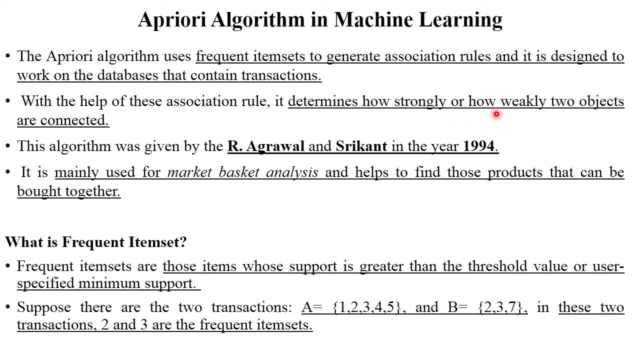 rules and if a particular thing, for example there is a milk and there is a laptop, so these two kind of items not purchased together. so this is called as weakly connected, right. so that's why this a priori algorithm are used. they check that whether the strong relation is there between 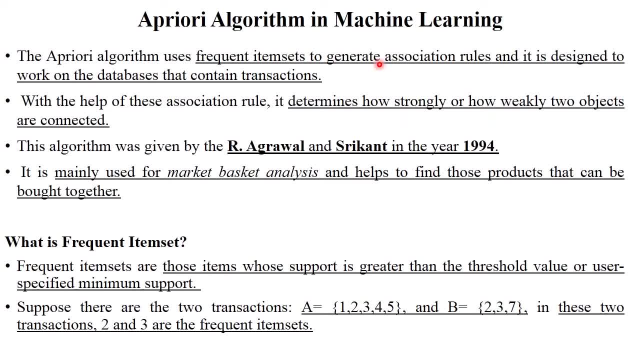 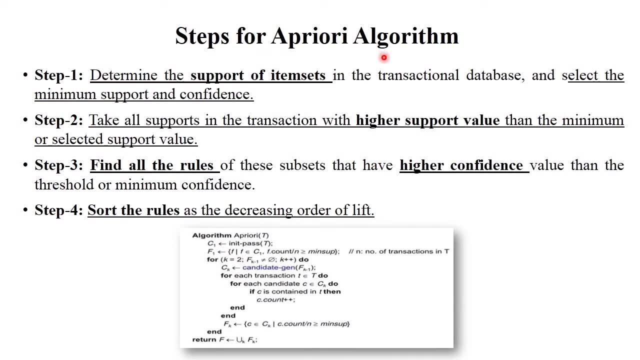 these two item sets, or weak relation is there. so that's why these algorithms are used, and this algorithm generally used in different market basket analysis. it helps to find those products that can be bought together. so let's see. so these are the steps of a priori algorithm. i will explain. 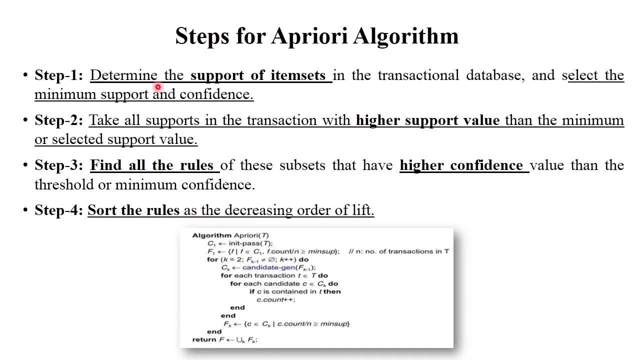 these steps with example. okay, so just review the steps. in step one, you need to calculate the support value as per your given data set. in second step, you need to calculate their confidence value, or highest support value. in third step, you need to find out the associated value of the product as per your given data set. in second step, you need to calculate: 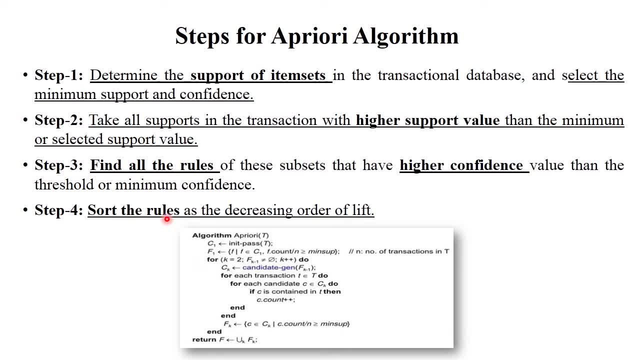 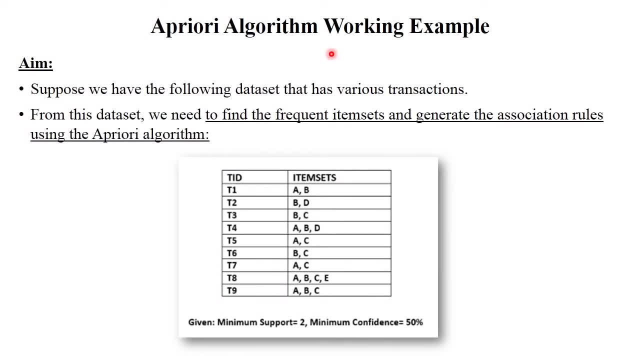 association rules and in step four you need to sort the rules. so i will explain these steps with example now. okay, so just see here. this is a priori algorithm working example. now. this is your given data set. okay, this is your transaction id and this is the item set, for example, the person one. okay, or? 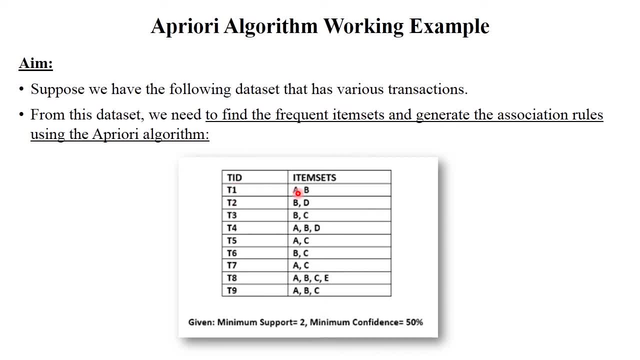 person a: this is your t1 transaction, so this person buy a and b item together. second person: that is transaction two. they buy a, b and b item. transaction three means person three by b and c item in this way. okay, so how many persons are there? there are total nine persons, mean nine transactions are there. 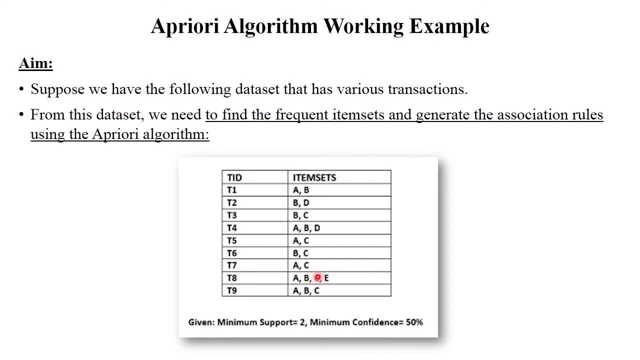 right, and these are the buying items, or purchasing items. now, here in your problem statement, support and confidence values are given. minimum support is equal to two and minimum confidence is equal to fifty percent. this is your given items. okay, so you need to find out which is your given items. 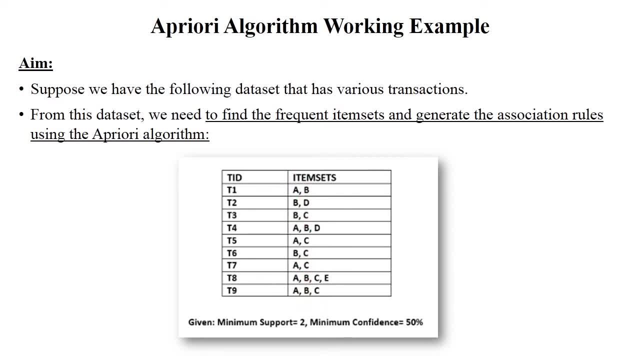 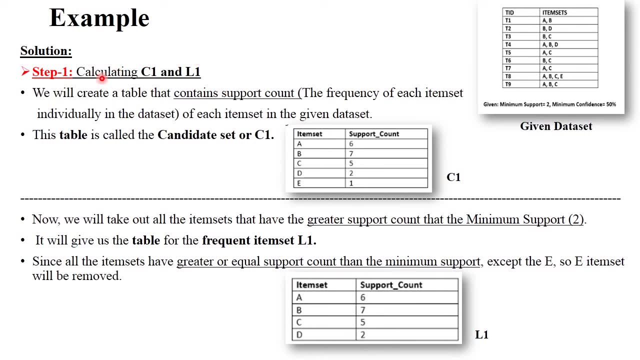 which is the best relationship or best association rule for purchasing the items. this is your problem statement. so next, okay, now the first step is you need to calculate c1 and l1. so what exactly it is? c1 means candidate set and l1 means frequent items set. let's see here. suppose this is your given data. 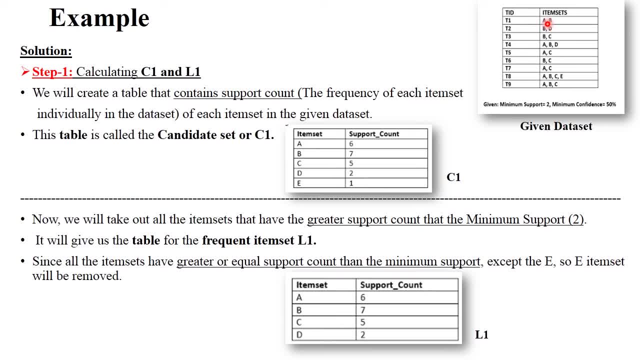 set. okay, how many items are there? total five items: a, b, c, d and e. total five items are there. here we are are there. okay, see here. this is your c1 table. there are two columns: item set and support count. you need to calculate support count in c1, so item sets are a, b, c, d, e. total five item sets are there. 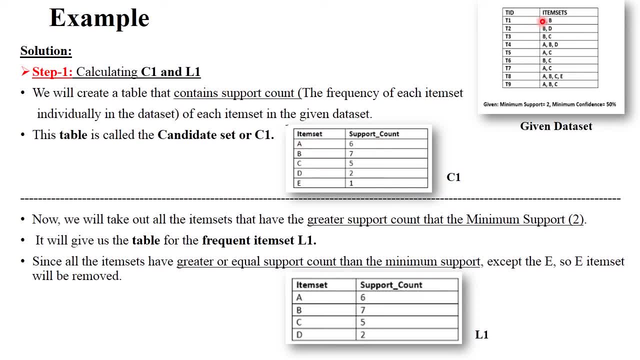 now how many times a item is purchased. so 1, 2, 3, 4, 5 and 6, so a items are purchased six times. similarly, b items are purchased seven times. c items are purchased. have purchased five times in this way. so this is item steps and this is support count. support count means how many times. 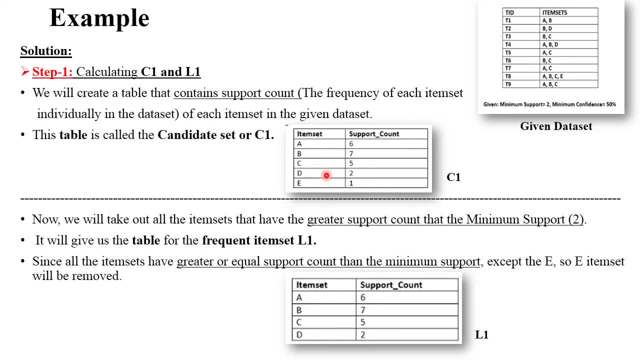 a particular items have purchased, right. so this is your c1 table now in l1 table. so in l1 table in your given data set, minimum support is 2. so as per your this c1 table, see here which is: minimum support is 2: 2, 5, 7 and 6 means 2 or more than 2, right? minimum support is 2, so you need to remove. 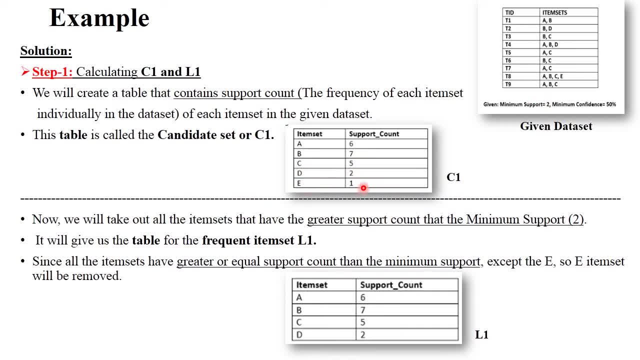 this item in your data set, that is e and support count 1. okay, so after applying minimum support, 2 is generated. the l1 table: see here. remaining items are as it is. just remove this thing, because this is not suitable to your given statement, because minimum support is equal to 2 only, right. so this is your l1 table, clear. 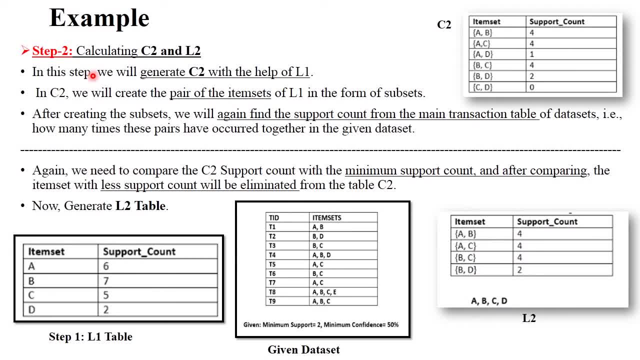 next, in step 2, you need to calculate c2 and l2 value. okay, now, what exactly c2? see here. so for c2, you required your previous c2 and l2 value. okay, now, what exactly c2? see here. so for c2, you required your previous. 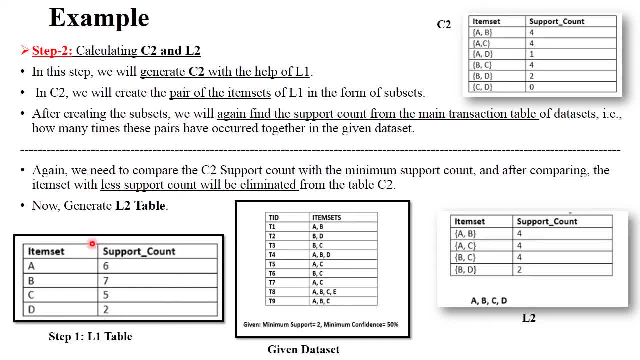 l1 table in step 1. okay, see here, this is your previous table. now you need to calculate how many times items are purchased together, for example the relations between this. for example, a and b items together, b and c items are together. see here: first a to b, a to c, a to d, then b to c. 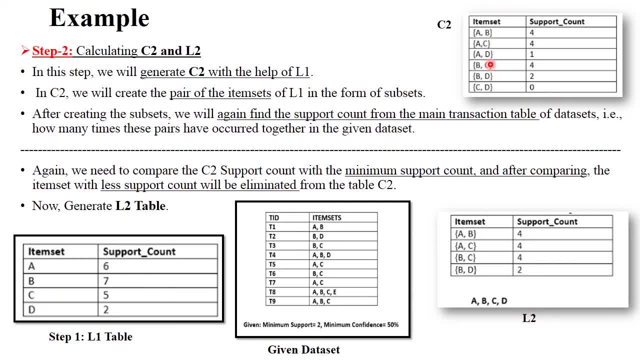 b to d and c to d. so you need to mention relation, two items, relation between that. okay, and now calculate how many times these items are purchased together. so you need to calculate how many times items are purchased together, for example a and b. so a and b items are purchased together, one, two, three. 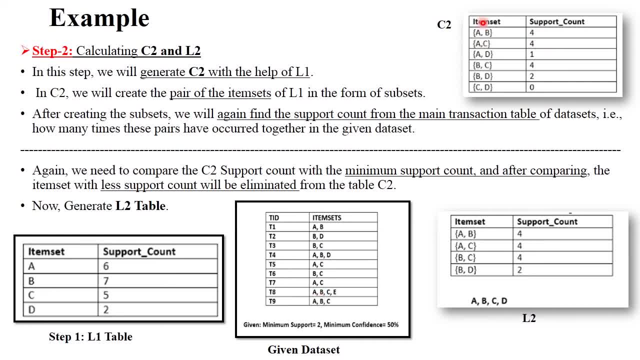 and four times in your given data set, similar remaining items are purchased in this particular time. okay, this is your c2 table. now again, your minimum support is 2, right? so according to this c2 table- you need to just take- minimum support is 2 means 2 or more than 2. so for this relation, 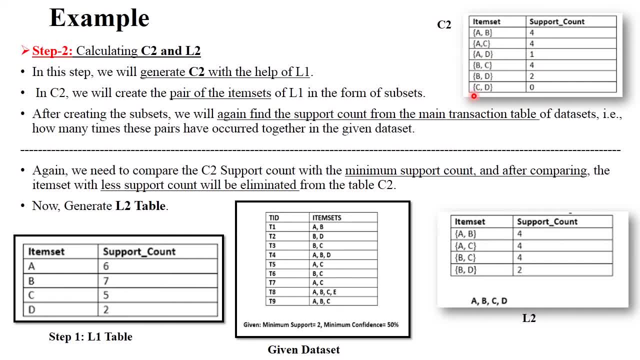 ad equal to one support count- this item purchase only one time- and cd equal to 1 support count, then equal to zero- this item purchase zero time. so you need to remove this thing, because minimum support is two, and just take remaining items as it is. so this is your l2 table. okay, next right, the next. 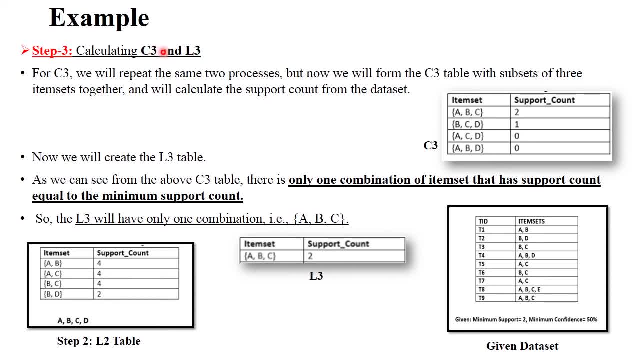 point is calculate c3 and l3. now three. three means three items purchased together. okay, now this is your previous table, l2 table in step two. so according to this table, you need to generate this c3 table. okay, so see here. first relation, three relations together: a, b, c next, b, c, d next. 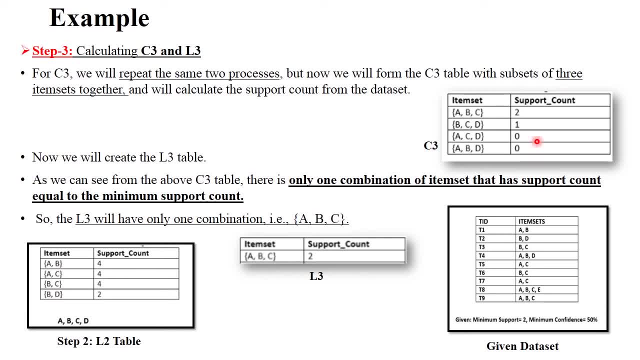 again: a c, d and a b d. so this four relations or four item sets are generated here right now. just check that these item sets in your given data set how many times a, b and c these items are purchased together. see here: a b c and a b c means these items are purchased together two times right. 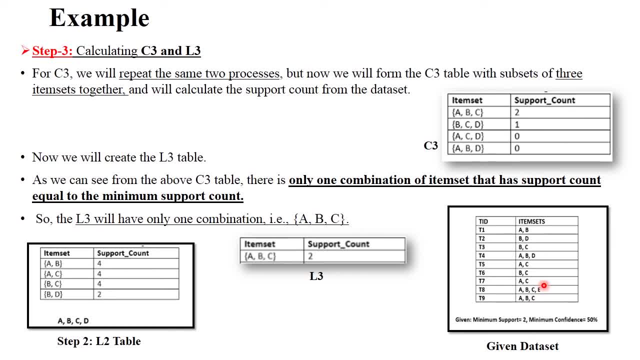 right now check b c d. so b c d. where is b c d? so see here b c and d. so these items are purchased together only one time. right and remaining: a c, d and a b d. these items purchased together zero times, clear. now again check that your minimum support is two. so minimum support is two, is here and remaining. 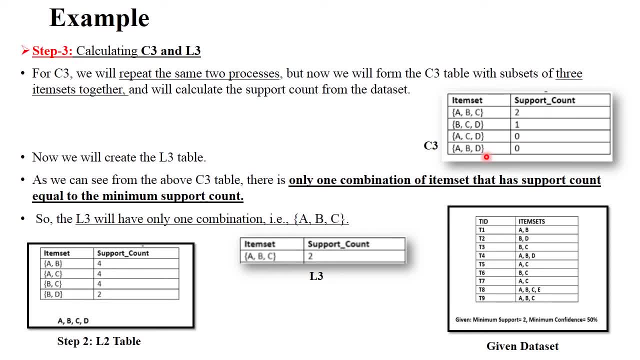 below two. that is one zero, zero. you need to remove these items. okay, so in l3 table only one item set is equal to two. okay, so this is your only one combination means item a, b and c. these items are frequently buy together. okay, next, now in step four, you need to find out the association rules. 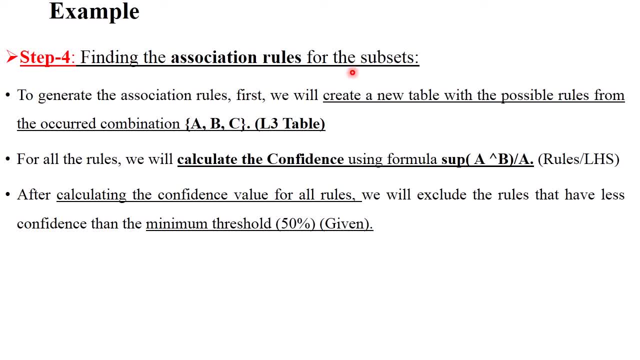 of the subset. in step one, two and three you just use support formula, right? you calculate the support of each and every items and the relations of each and every items. now, in this step, step four, you need to calculate association rules. so, as per your previous step, a, b and c, as per your l3 table, these combinations are generated, okay. 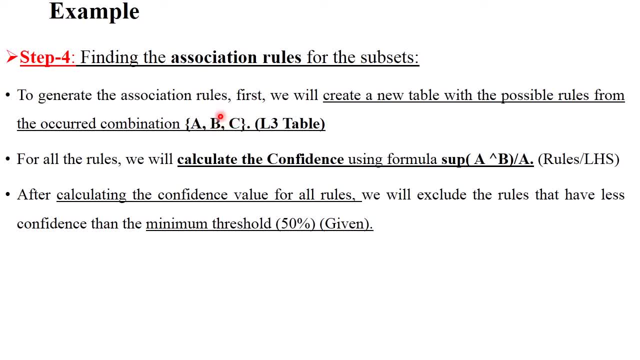 now you need to calculate the association rules between this a, b and c. so for that purpose you need to use confidence formula, and confidence formula is this: support it. it is to b upon a. this is a formula of confidence and in your data, given data set, minimum confidence value is 50 percent. 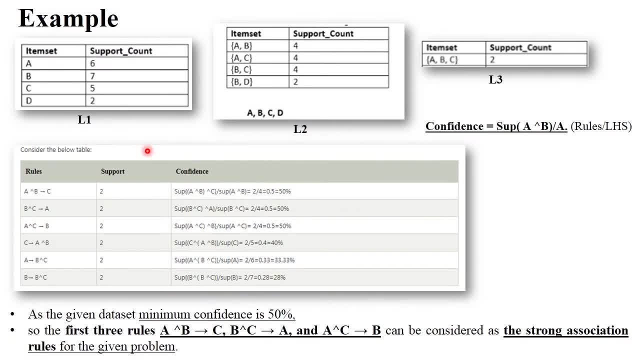 so let's see the next right now. see here: this is the step, your step four. so in step four, there you need to generate this table. okay, the first is rules, second one is support and third one is confidence. so here, rules and support, these are items are already generated in step one, two and three. now see here. so, uh, as per your given. 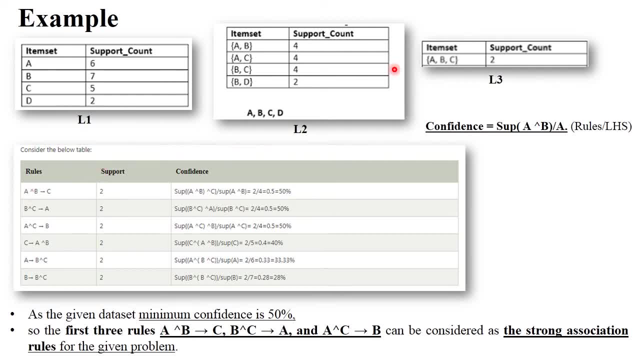 relation: previously a, b and c. this is your given relation right as per your l3 table. these three items are frequently buy together. now just make a relationship between these three items. see here. these are the association rules, for example, a, b to c, next b, c to a, see here. next a, c to b. next rule is c to a to b, then b, a to b to c. 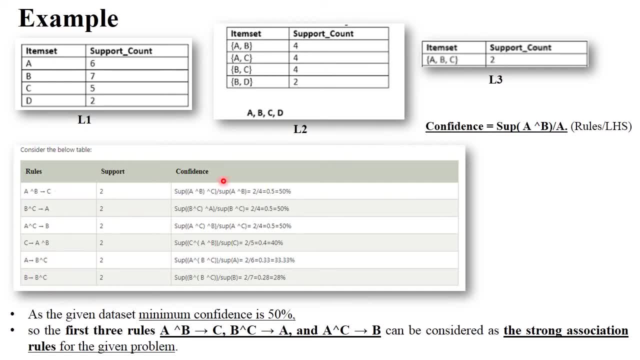 and b to b to c. so these six rules are generated as per this given item set. right from this three item set, six rules are generated. and now let's check their support count. is here, for example, a, b, c support count is two. is here now b c, a, b c, again same b c, a support count is two. and in this way, 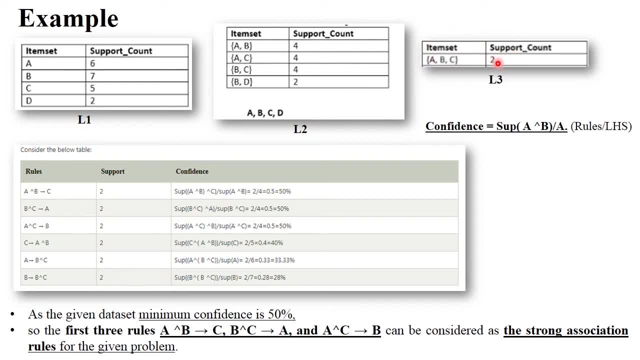 the complete item set support count is two because this item purchased two times. so that's why the support counts are two. now next one is confidence formula. see here rule divided by lhs. so the first: you need to calculate confidence of this rule. how to calculate? see here support and mention these rules. are there support here to b to c? so you need to. 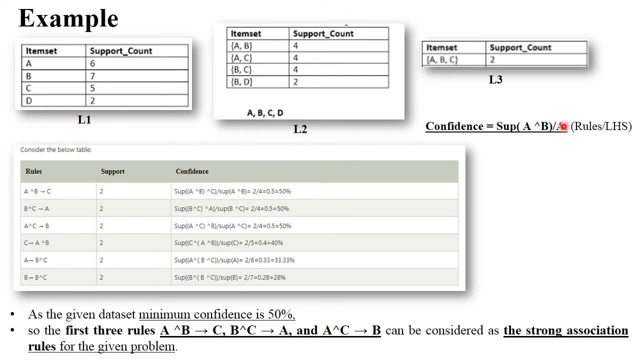 mention this rule divided by lhs or a. so your lhs is this: support a to b. this is your lhs. this is your rhs, right lhs to rhs. summation divided by lhs. so that is support a to b. so just see here what is the support of a, b, c, support of abc is two. so two divided by support of ab and support of ab is four. 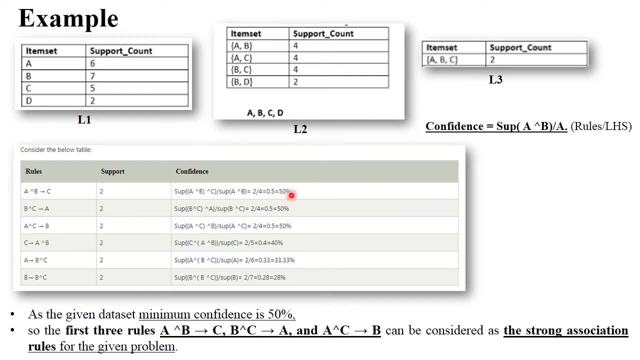 so two by four, zero point five, it is fifty percent. now fifty percent chances are there. when person buy a and b item, then they buy see item also. so fifty percent chances are there. now next b, c and a. again same support of b, c, a divided by support of lhs. 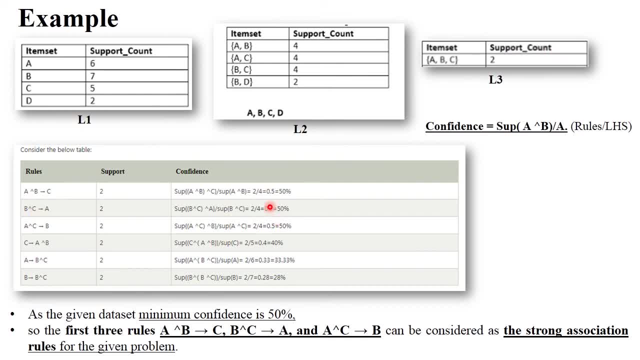 support of b c. so b c a support count is two divided by support of b c is four. so two by four again fifty percent. so in this way you need to calculate the confidence formula upto last of every rule. now in your given data set, minimum confidence is fifty percent. 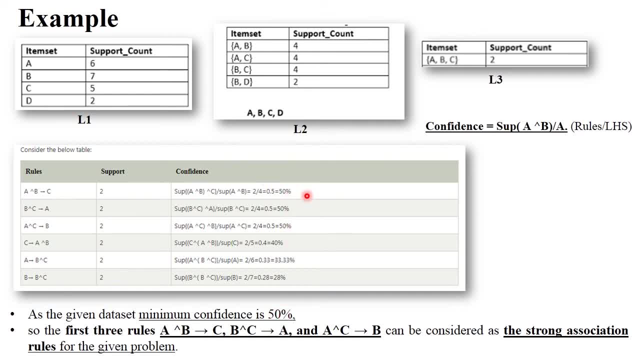 so change this. your given confidence chart check here. minimum confidence is 50% means rule 1, rule 2 and rule 3. these three rules having minimum 50% confidence are there right. so these are the strong association rules. you need to remove these three rules because that is. 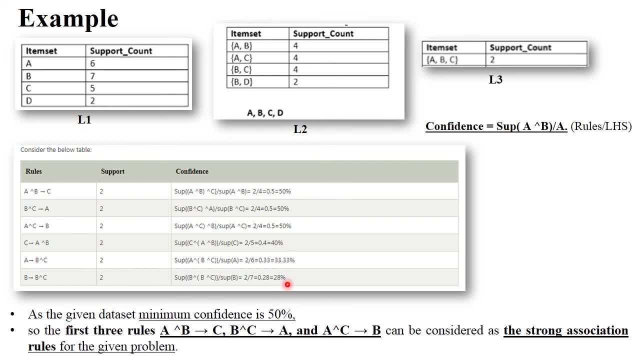 minimum or 15%, not a minimum 50%, right? so just focus on these three rules, because minimum confidence is 50%, as per your given data set. so when person buy A and B item, then they buy C. when person buy B and C item, then they buy. 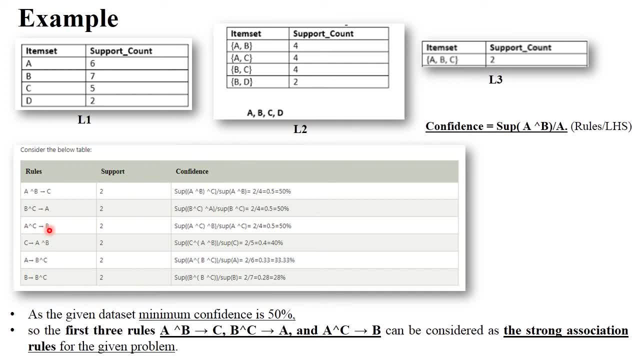 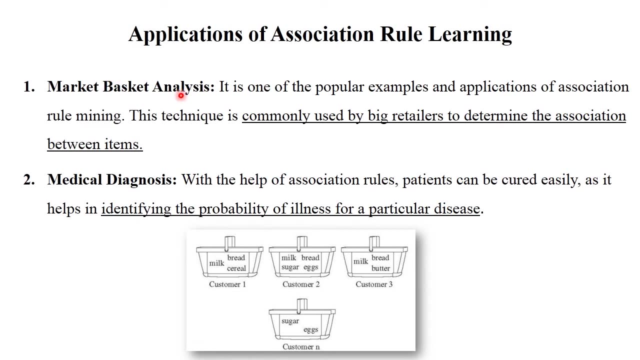 A, and when person buy A and C item, then they buy B also. so these are the strong association rules. in this way, a priori algorithms are used to calculate the association rules in market basket analysis purpose. now next, applications of association rules. so, as we discussed, market basket analysis is one of the